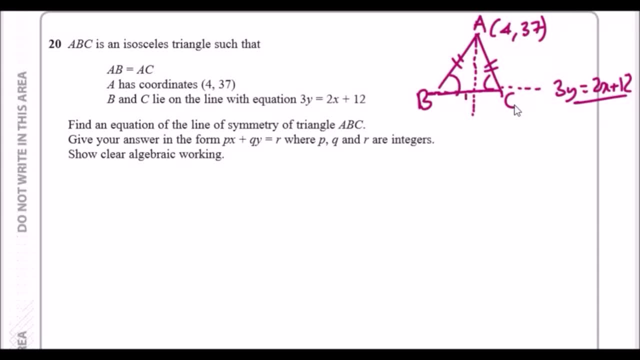 and yeah, just quick note. if this is a line of symmetry, that means we have two perpendicular lines, So that could be useful for a second. Give your answer in the usual form: All right, cool, So let's do this. So what can we? how do we start with this? So what I would, personally? 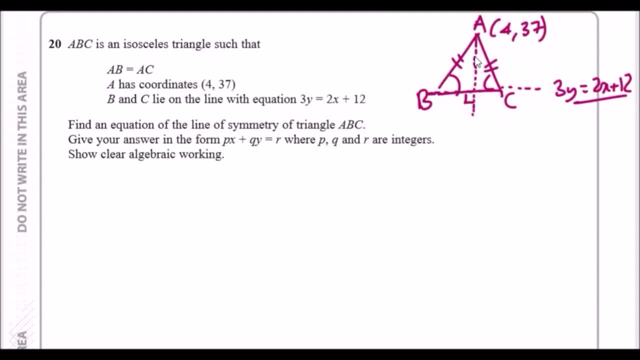 advise that since we've got a coordinate here which is on this perpendicular line and we've got a line already here, we should go ahead and find a gradient of this line, And to do that we need to rewrite this in the usual y equals mx plus c form, where m is the gradient. 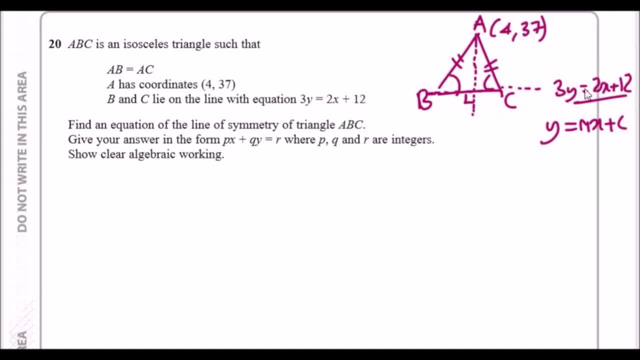 Okay, so we're going to go ahead and find the gradient of this line, And to do that we need to rewrite this in the usual y equals mx plus c form, where m is the gradient. So so far, it looks to me that it's almost there, which we just have to divide this equation. 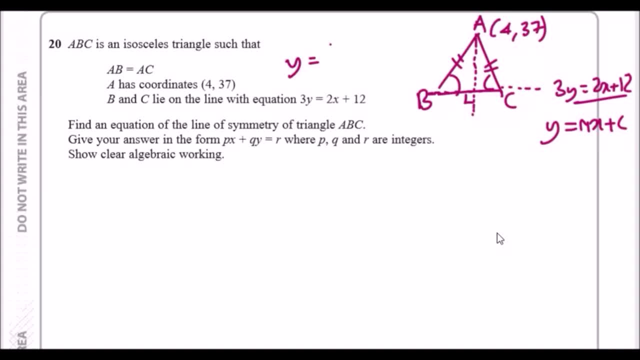 by three. So we're going to have y equals two over three, x plus four. So this means the gradient of the line that cuts through BC is two of x, but the perpendicular gradient of the line from a downwards is going to be the reciprocal negative, the negative reciprocal. 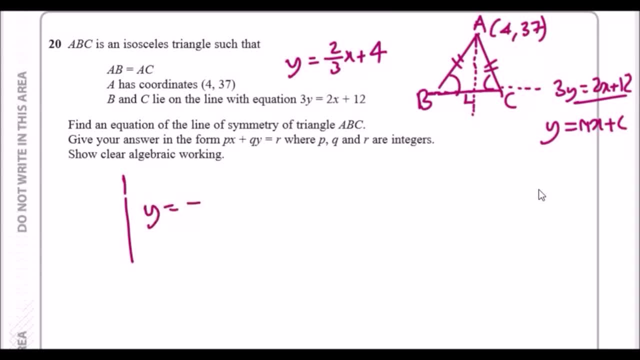 So we can say that the line going downwards is going to be y equals minus three over two, x plus something which we don't know yet. So we actually almost there was literally just go find C. But it's easy now because since we know that there's a chord on this line, that full phase seven. 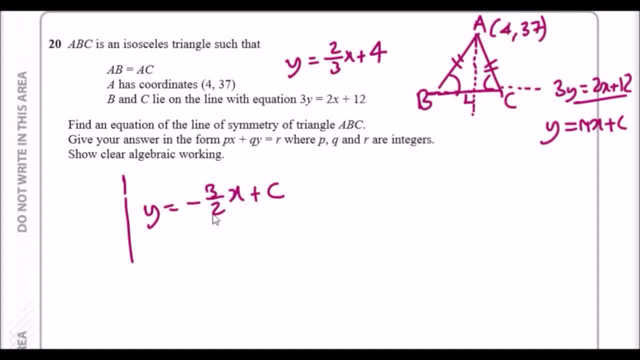 is on that line which is plug in: x is four And y is 37. So let's do that plug in in four, phase seven, when one ys 37. And x is four, So before times three over two, which is minus 12, over to plus C, then we: 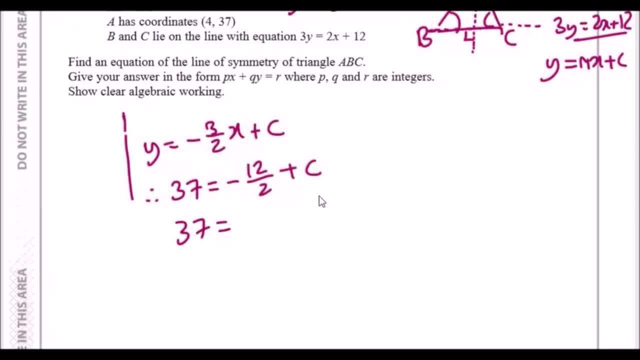 have a down. So minus 12 over two is minus C. Okay, we're going to go back to the middle of this. This one 6 plus c. so the purpose is is to find the c value, and then we can rewrite in that usual form. 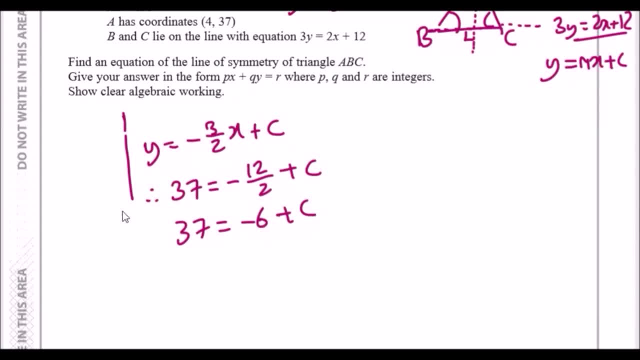 now we just add 6 across, which is going to give us 43 and yeah, that's our value for c now putting it back in the usual form. so we've got y equals minus 3 over 2x plus 43 and the form they want.